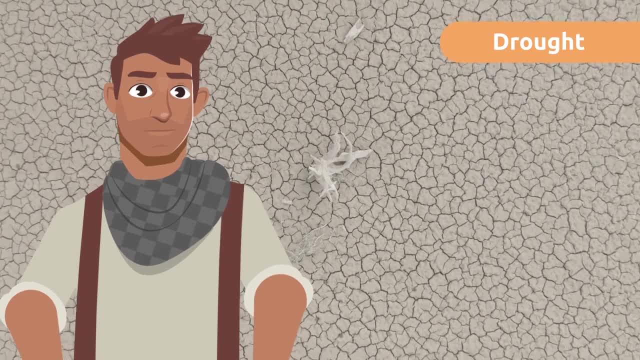 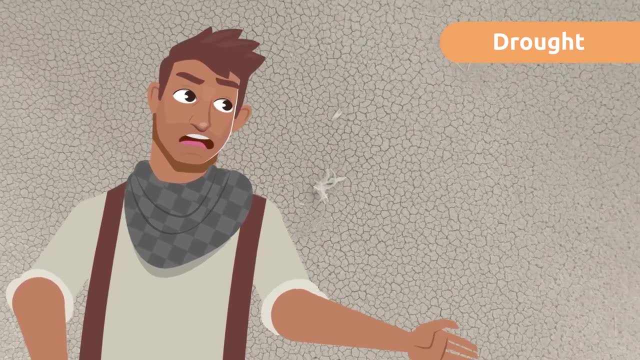 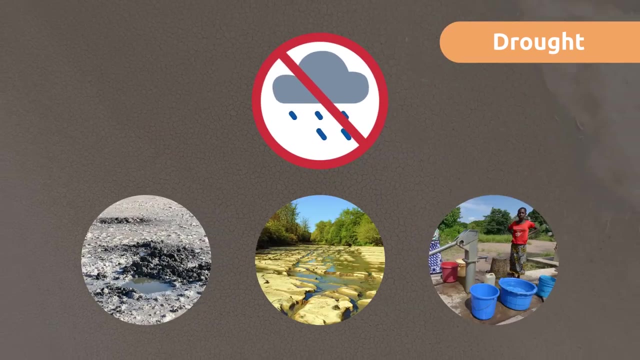 than usually available in a given area for an extended period of time. Unfortunately, droughts are an increasingly common phenomenon, Due to the fact that rainfall is less frequent than in previous years. this means that rivers, lakes and wells have significantly less water. When there's a drought, there isn't enough. 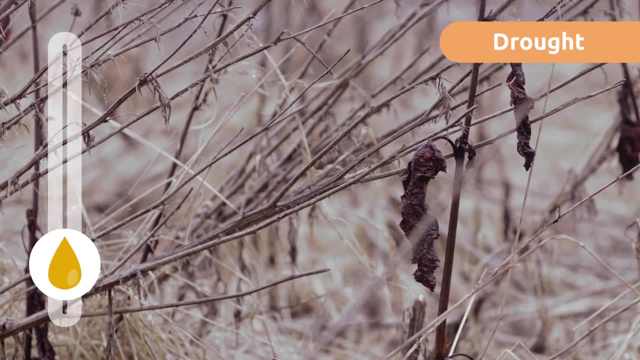 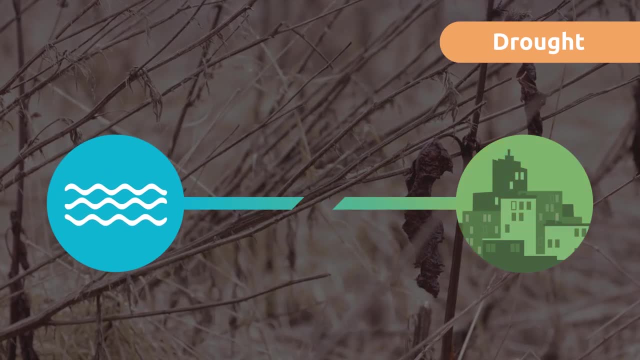 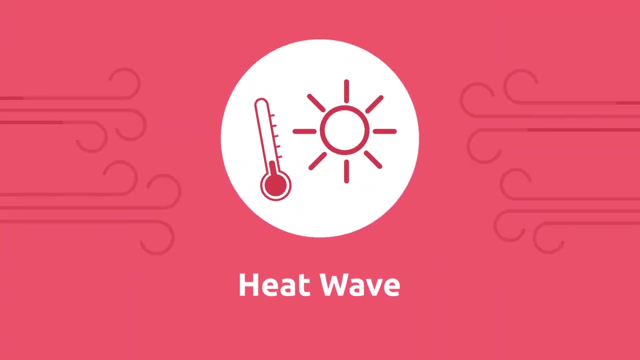 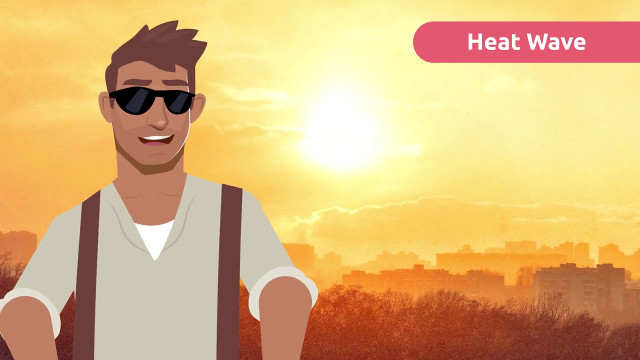 water to irrigate crops, so plants die as well as the food they produce. During periods of drought, water shortages can also occur in populated areas and, as you can imagine, it can cause major problems for the local residents. Heatwave: A heatwave occurs when the temperature in 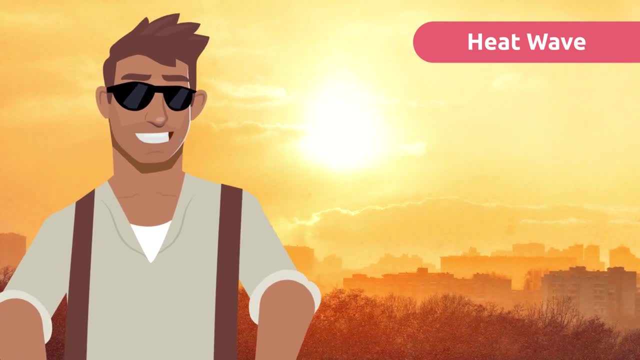 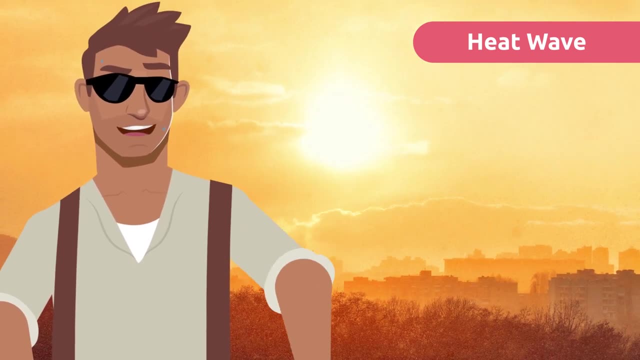 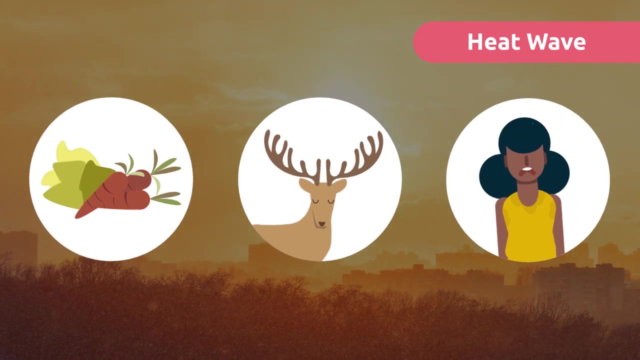 a given area is extremely hot. Normally, this phenomenon takes place in summer and usually favors a drought. Ugh, it's so hot. Heatwaves are detrimental to living things in the area. Crops spoil, animals and humans can become dehydrated. 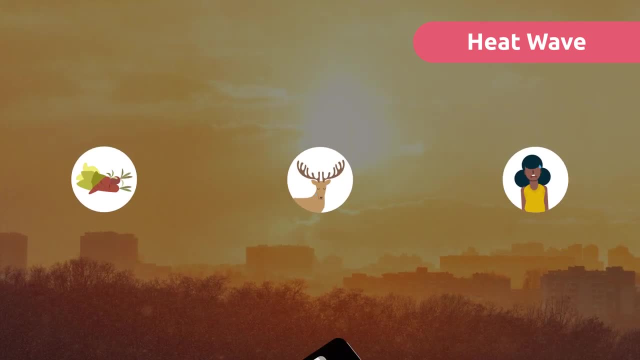 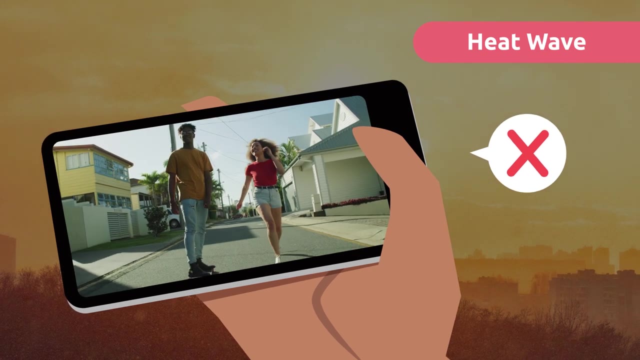 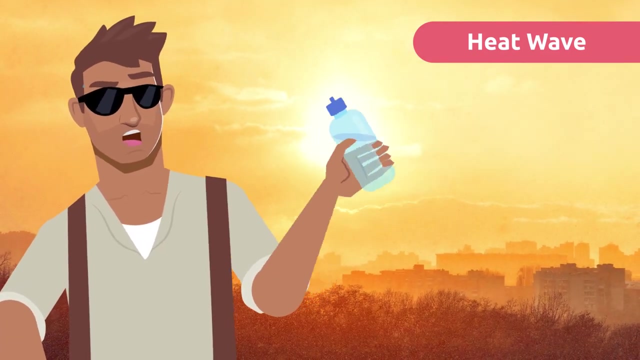 Never underestimate a heatwave. During a heatwave, it's recommended to stay in shady places or under coverings, Don't go outside during the middle of the day and avoid intense outdoor exercise. So make sure to drink plenty of water and stay in cool places. 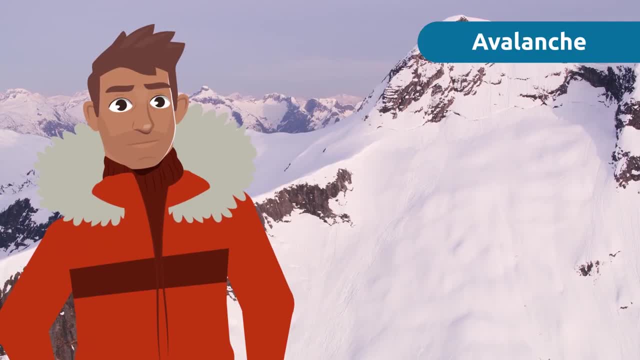 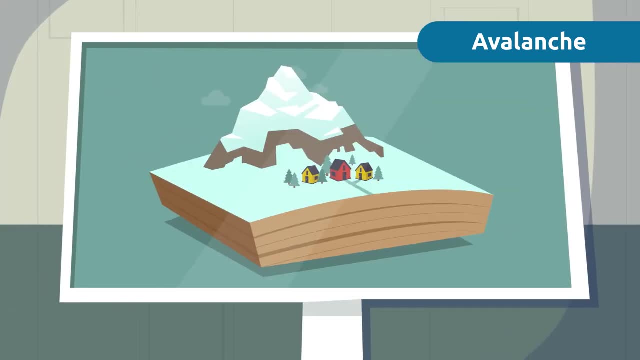 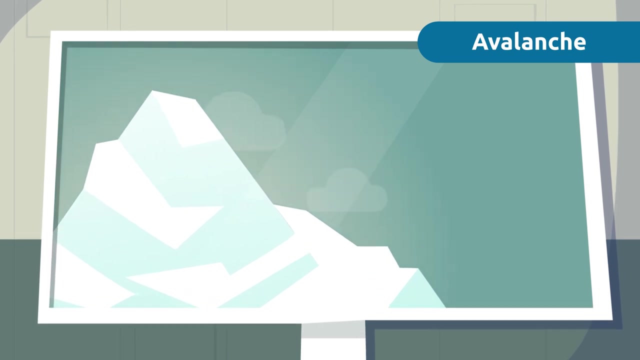 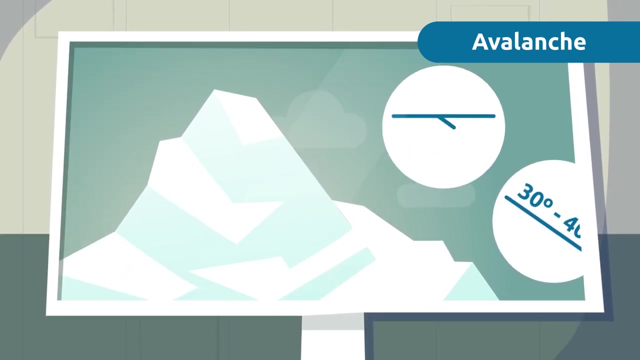 Avalanche. A avalanche usually occurs in mountainous areas. It's a huge mass of snow that suddenly slides down a mountainside at high speeds. To trigger an avalanche, there must be an unstable pile of snow and an inclination of between 30 and 40 degrees. A pile of snow can fall off due to gravity or simply an animal's footstep. 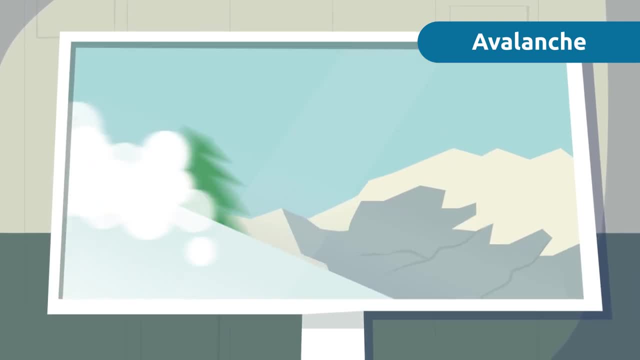 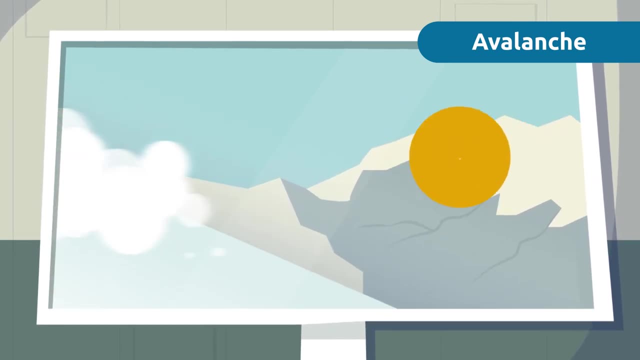 These are some causes of an avalanche. An avalanche can reach a speed of descent up to 186 miles per hour. An avalanche can reach a speed of descent up to 186 miles per hour, Sweeping away everything in its path. Avalanches increase in size during their journey because 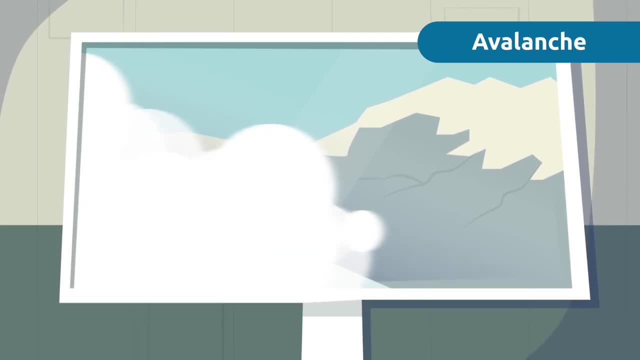 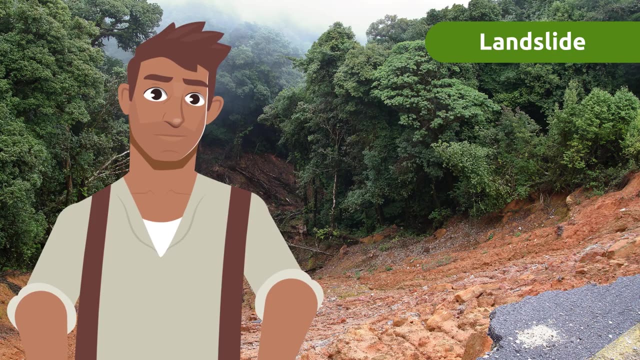 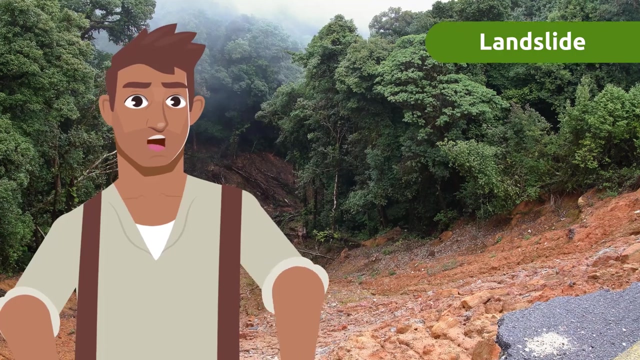 it not only includes snow, but also vegetation and rocks. Landslide? A landslide is the movement of a large mass of earth or rocks sliding down from higher elevation to a lower elevation. Landslides can be caused by different reasons, such as heavy rains, earthquakes or snow. A landslide? 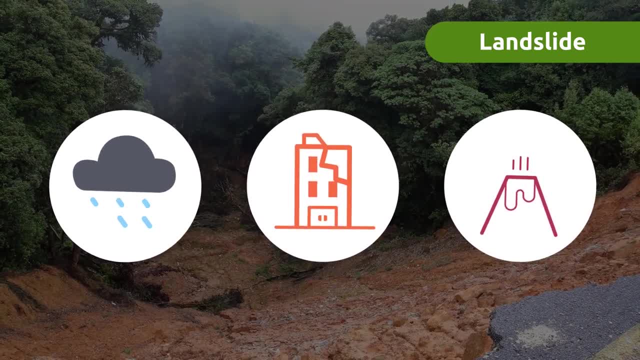 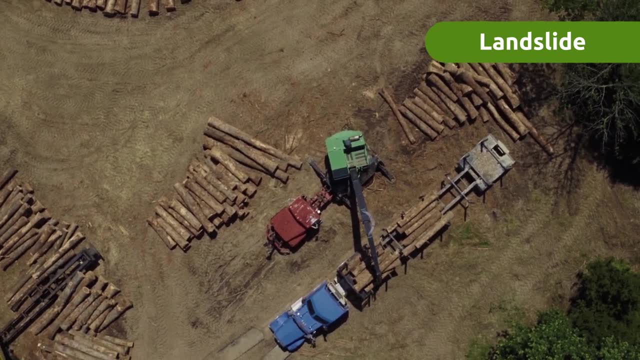 can cause landslides to be caused by heavy rains, earthquakes, volcanoes or simply by unstable terrain. Like in other natural disasters, human action can intensify the severity of this phenomenon. Deforestation is one of the triggers When there are no roots to help. 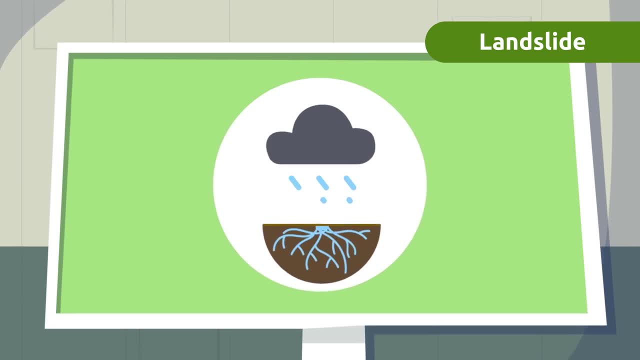 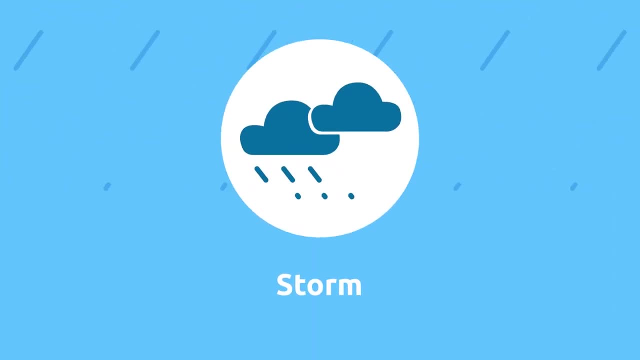 hold the soil components together, the ground becomes wet due to rainfall and these land shifts occur: A storm, Storm. A storm is a direct reaction to a monsoon. A storm becomes a response to the event of a monsoon. A storm is a direct reaction to a monsoon. A storm is a direct reaction to a moment. 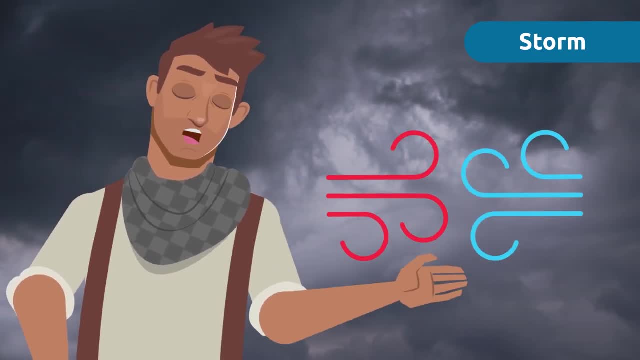 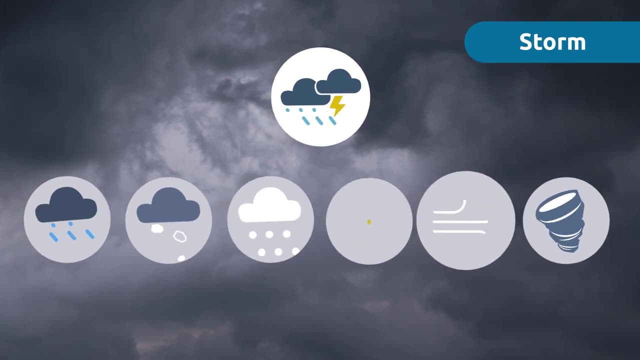 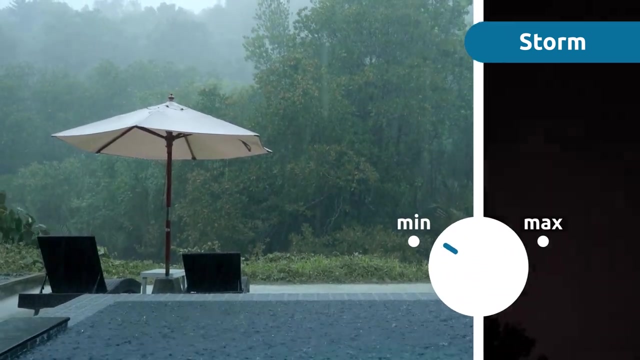 happens when two air masses of different temperatures and pressures collide, giving rise to phenomena such as rain, hail, snow, lightning, strong winds or even tornadoes. Storms can have different intensities. Sometimes they'll be very mild or very destructive. There are many types of storms, such as thunderstorms. 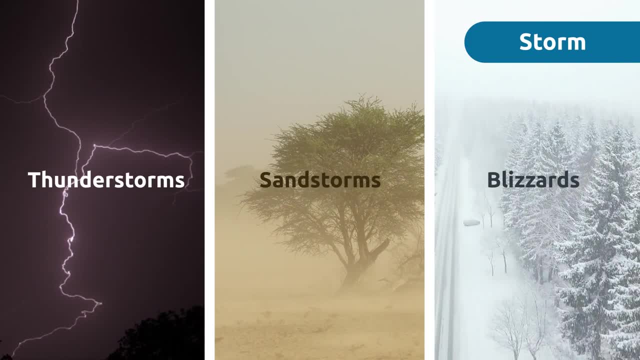 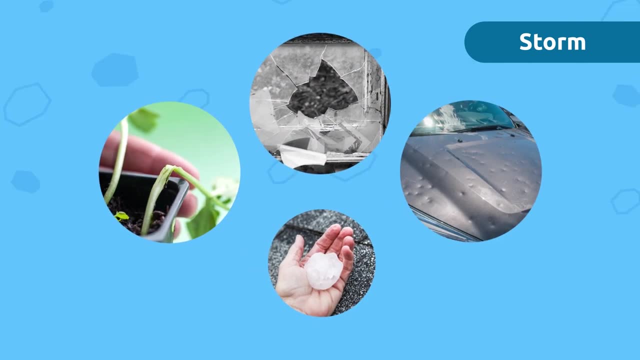 sandstorms or blizzards. There are times when storms produce hail, which are balls of ice that fall violently from the sky. Hail is very damaging to the environment. It destroys crops and it also can cause damage in cities, like breaking windows. 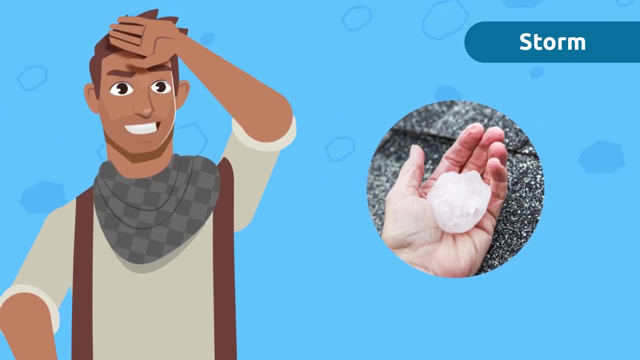 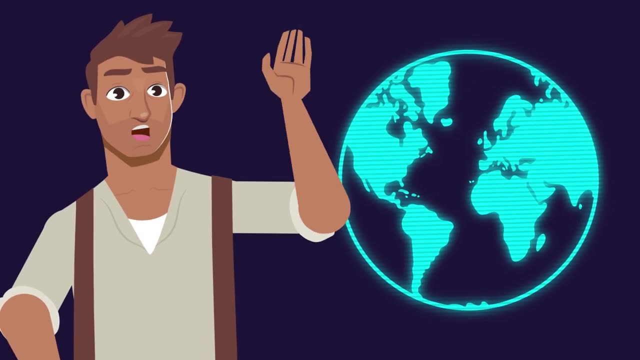 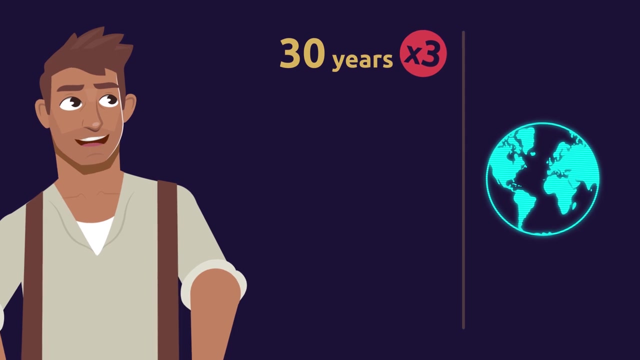 or denting cars. Make sure to take cover when it hails. If not, you might end up with a bump on your head. Finally, I'll give you some facts that you should keep in mind about natural disasters. Did you know that they have tripled in the last 30 years? Also, did you know that? 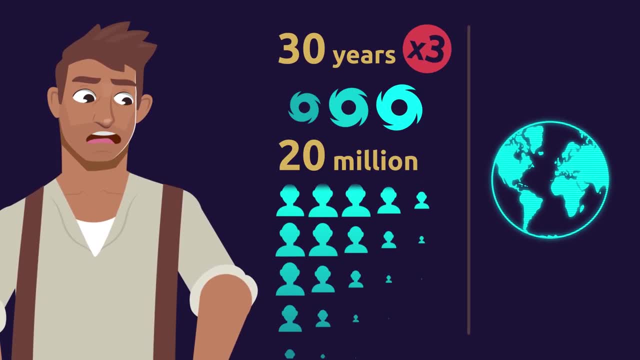 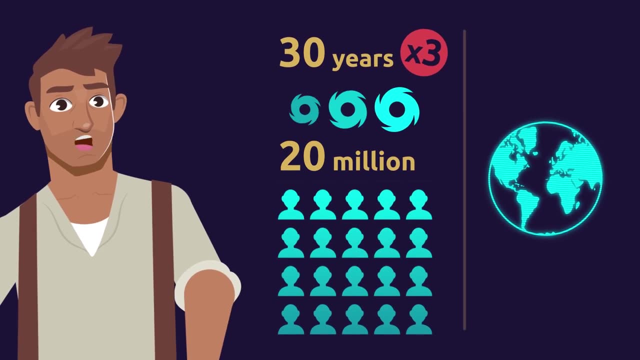 they are more destructive than ever and that 20 million people are forced to leave their homes every year because of them. Impressive, isn't it? A large part of this increase in damages is due to the Earth's increasing temperature. ie.